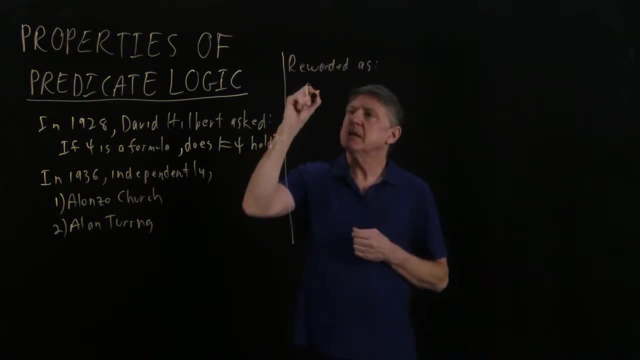 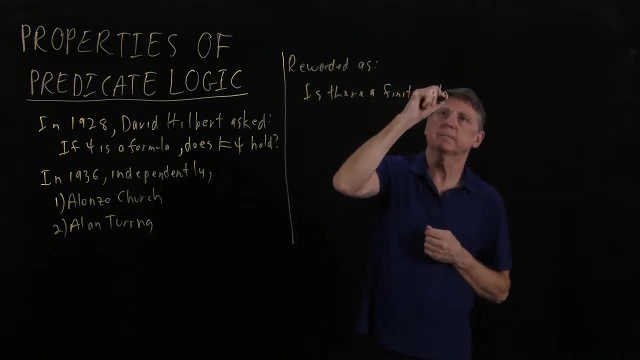 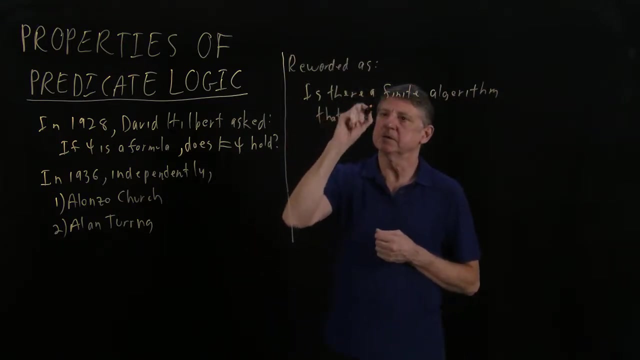 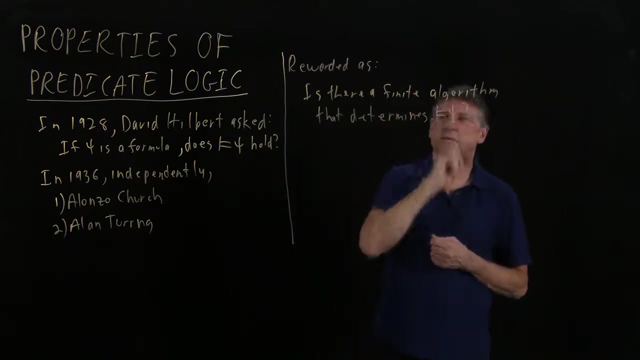 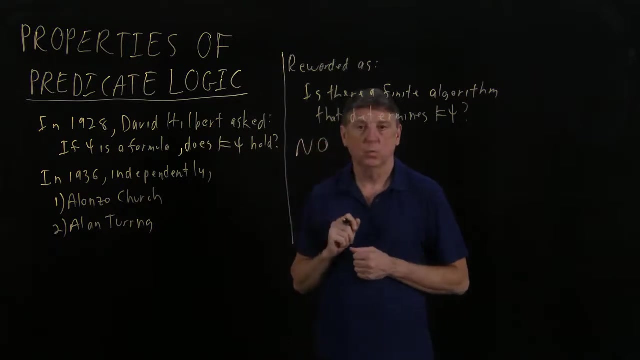 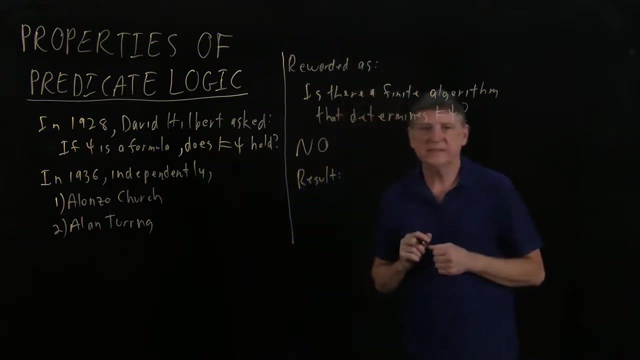 not technically Reworded as is Is Is, Is there a finite algorithm that determines whether a formula is valid? And their answer, remarkably, was no, And this means. So the result of this is we say not just a formula, but we say all of predicate logic. 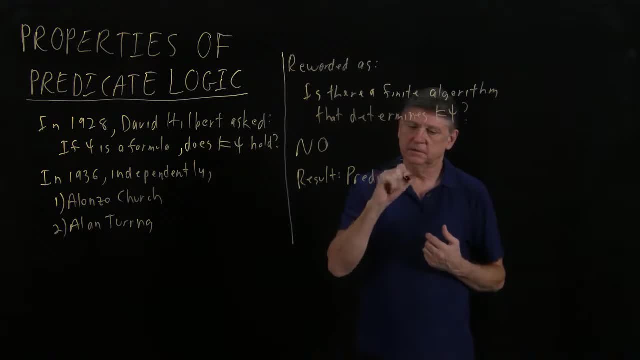 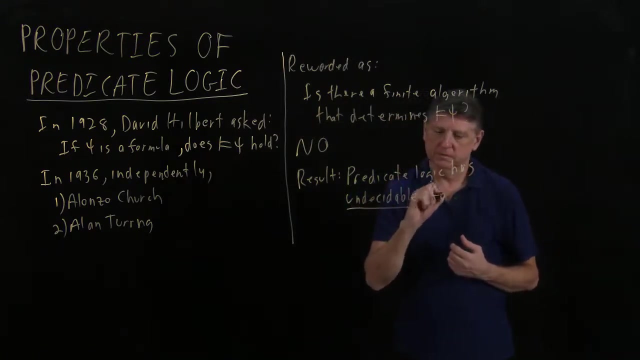 We say that predicate logic, I'll say, has undecidable, undecidable formulas, And in fact it has an infinite number. It's not just that there's one formula that's difficult, It's that there's an infinite variety of these. 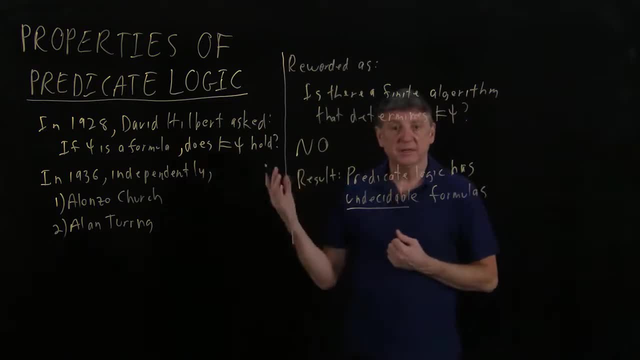 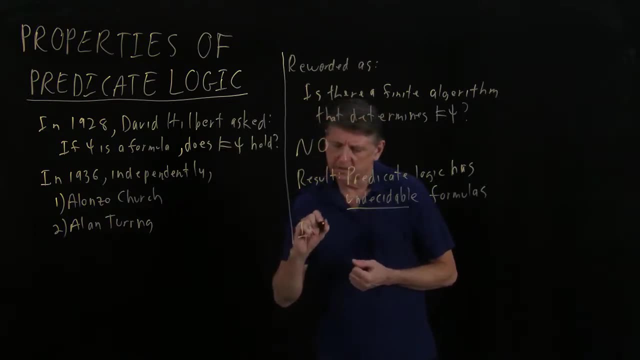 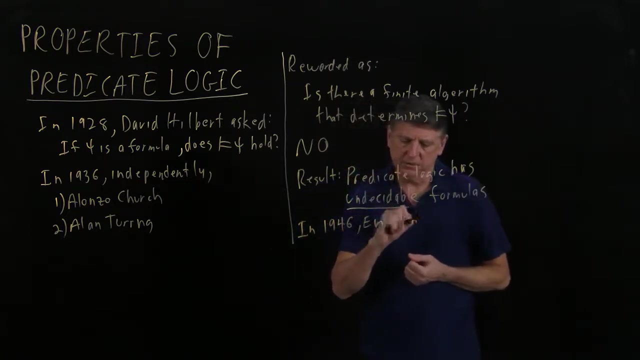 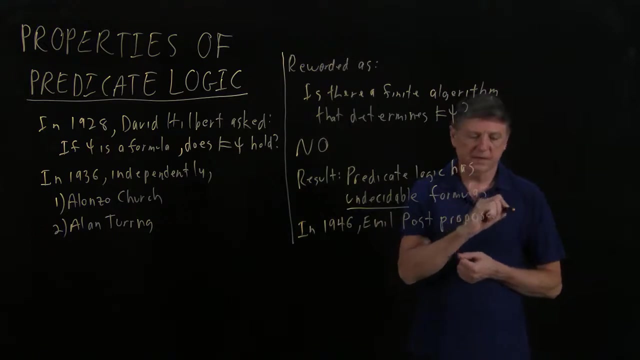 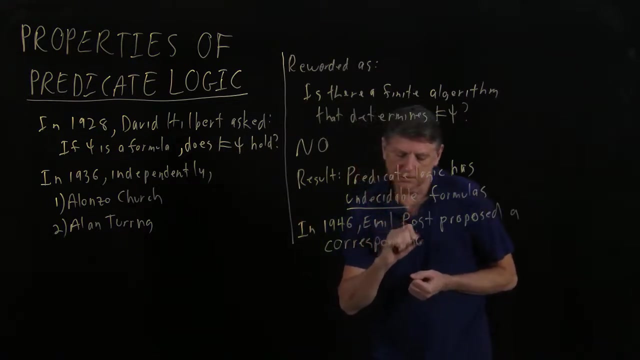 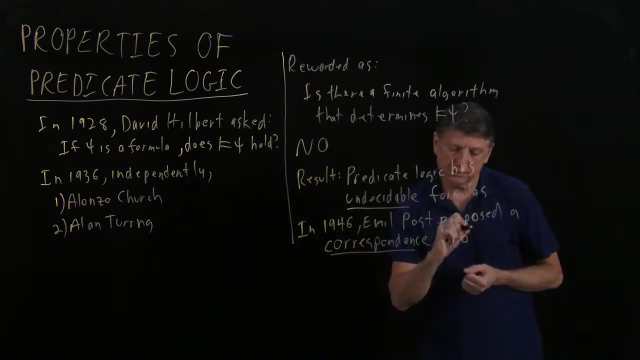 And one, one way that was illustrated much later- not much later, but later. This was in 1946.. E-mail Post proposed a specific example. E-mail Post proposed a specific example And he called it a correspondence problem. And this correspondence problem is, if you're really interested in logic, this correspondence. 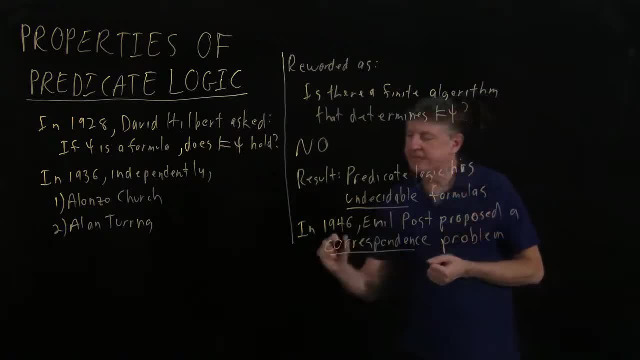 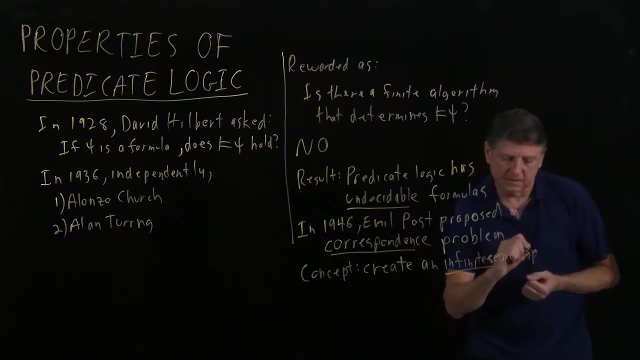 problem may be worth some further study, and the concept behind this is that what E-mail Post did? was he created? He created an infinite, infinite search space. that is he. what email post did was he found a finite problem that had an infinite search space that had to be checked, and 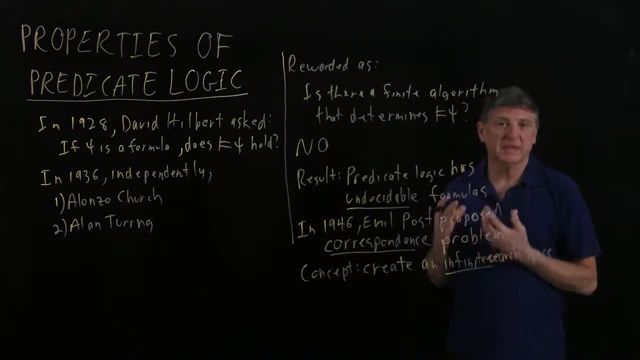 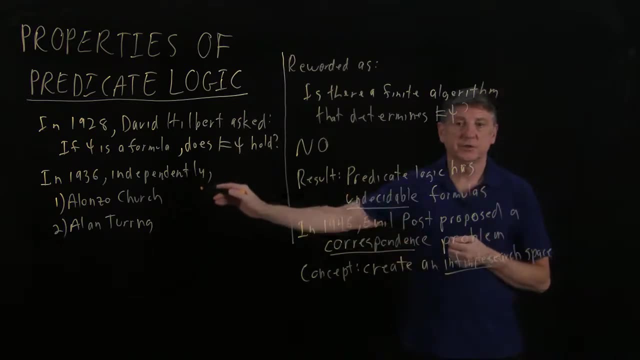 if you have to check an infinite search space, then you can't determine that with a finite algorithm. so in 1936 Church and Turing use highly technical arguments that demonstrated that Hilbert's thesis was false. that is, there is no algorithm for determining whether a formula can be proved or not in predicate logic and in